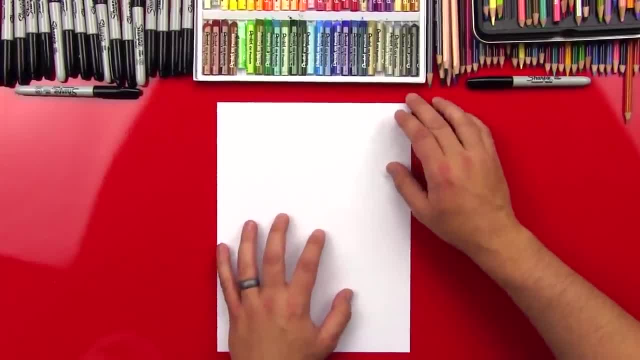 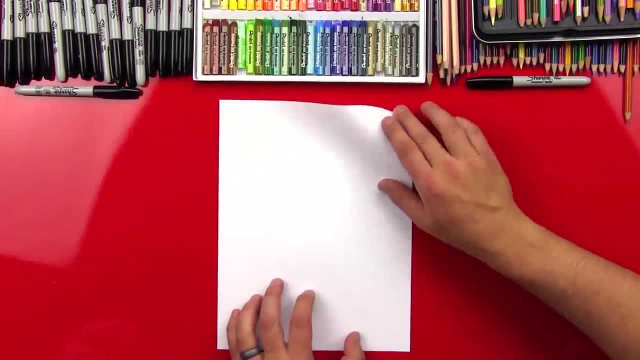 to fold it up to the top, okay? Or we can put it like this: Sometimes that's a little easier: We'll fold this corner down to this side, and so this edge is going to be lined up here and you're going to be my helper, right? So I'll line it up and then you fold it, okay. Okay, I'll get it down. 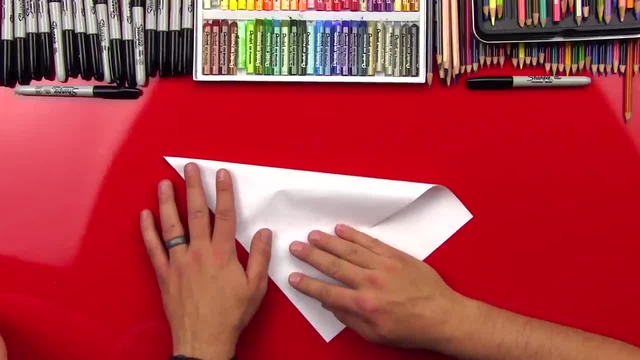 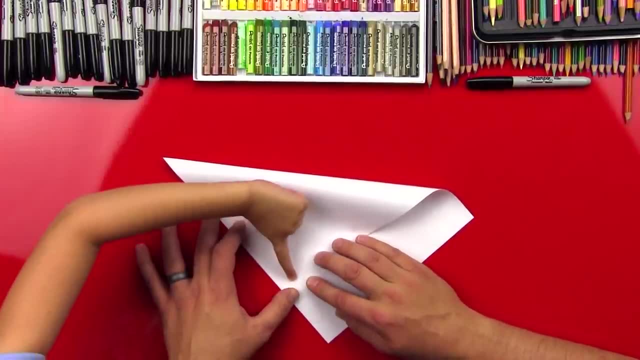 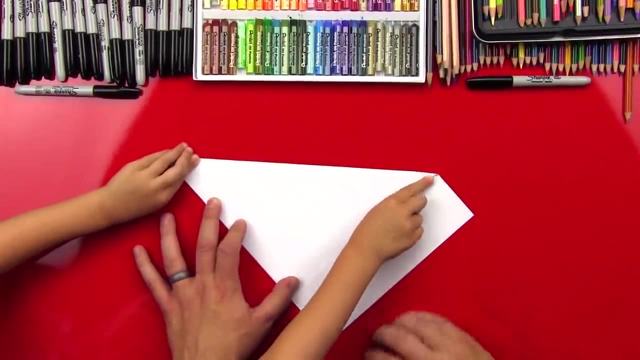 one second. Hold on, let me get it lined up. Make sure that there's a point up at the top Like that: All right, do your thing Right down the middle. I love how you fold stuff. Good job, Yes, Perfect. And we want to make sure that that's nice and crisp so we can take our fingernail down. 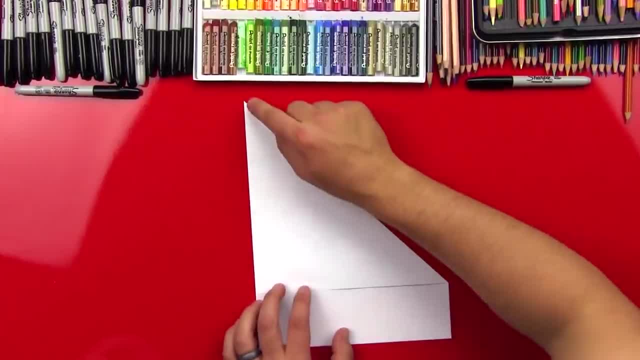 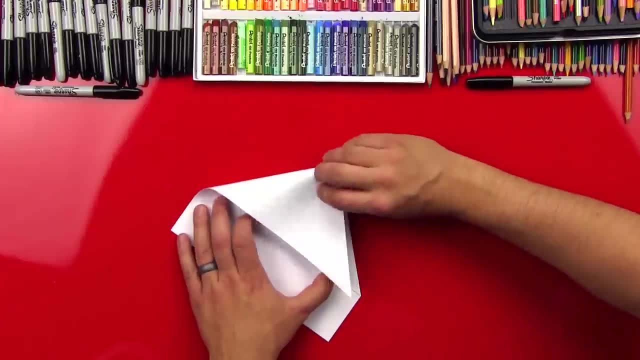 it a couple times too. Okay, now we're going to take this corner up here and we're going to fold it down to this corner, okay, And it's going to look like a little house. when we're done, We'll fold it. 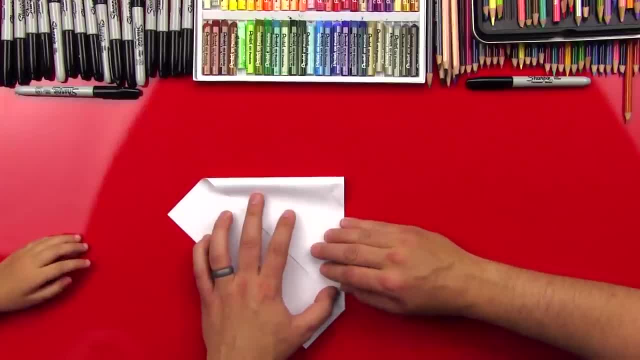 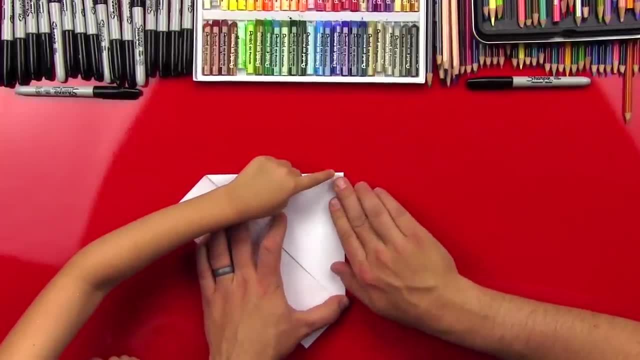 Fold that down. and this is a fun project, isn't it? We've done this before and it was so much fun. Okay, Sorry, I almost did your step. Okay, ready, Fold, Fold away. Good job, squeaky fingers. 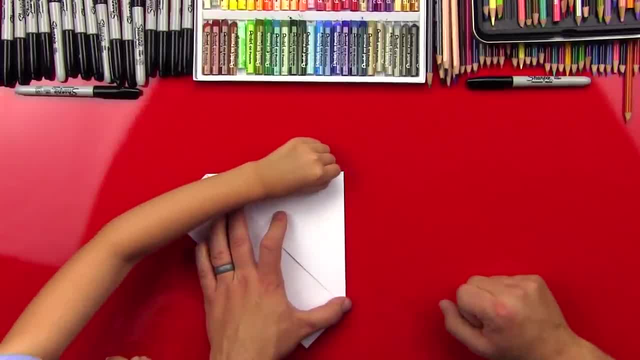 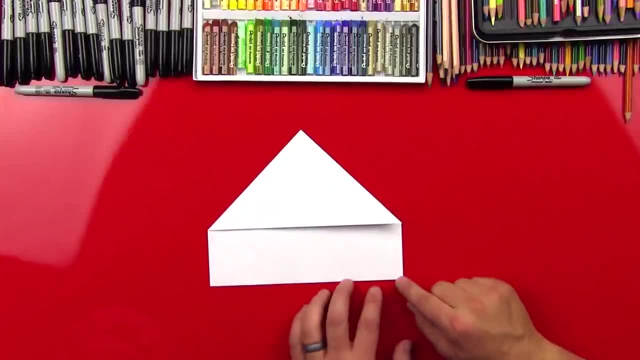 You did it, Good Yeah, and take your finger now and make it nice and crispy. Good job, little girl. Okay, now our next step, and this is why we don't want a square piece of paper, because we're going to take this. If we had a square piece, this piece would be missing. So we have this and we're. 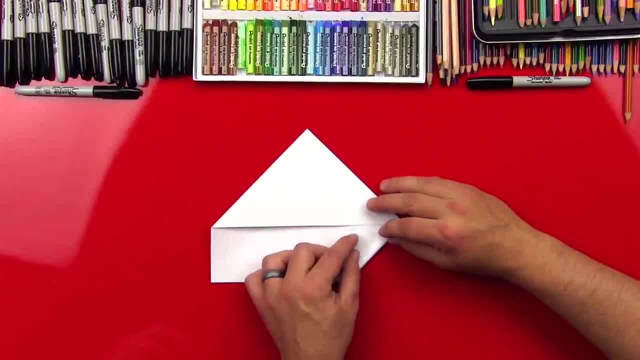 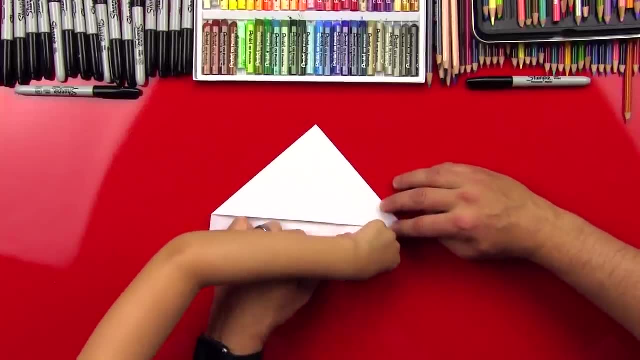 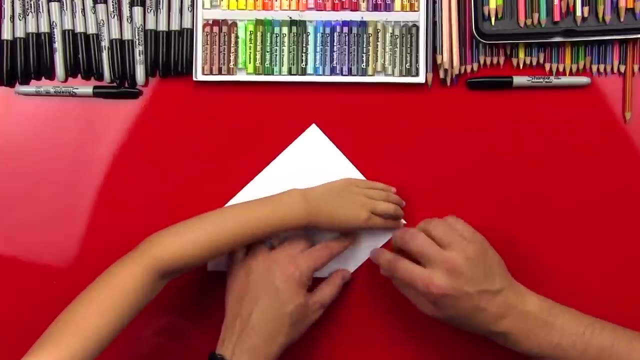 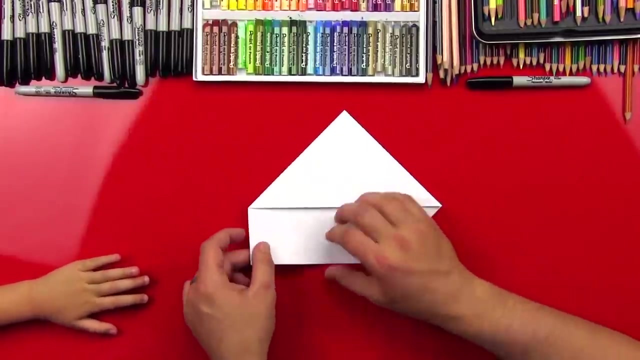 going to fold this corner up like this, to that line: Okay, fold away- Good job, Press it down- Good job, You did it, Okay. and then we're going to repeat that same step on the other side. Okay, so we're going to take this corner right here and we're going to fold that one. 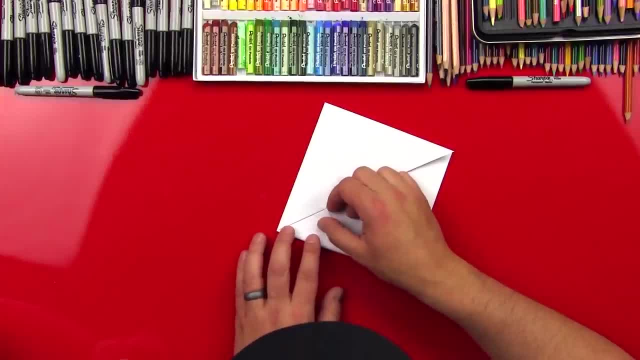 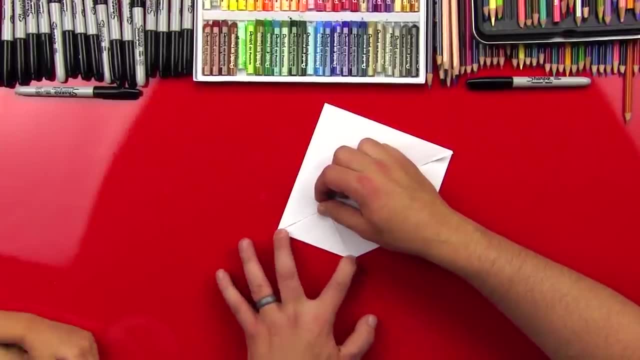 Up to here. You ready to fold it again? There you go: Fold down the middle and then up to the edges. Perfect, Did it? Okay? now we're going to take this bottom edge and we're going to fold it up. 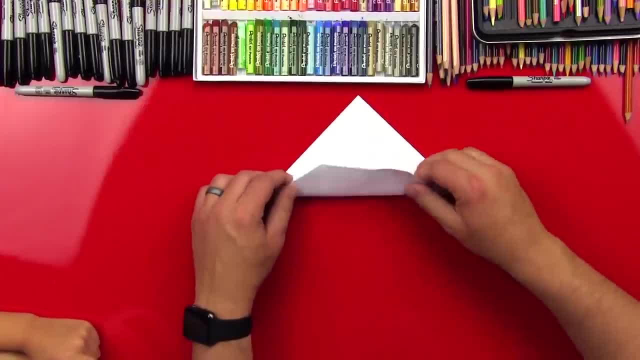 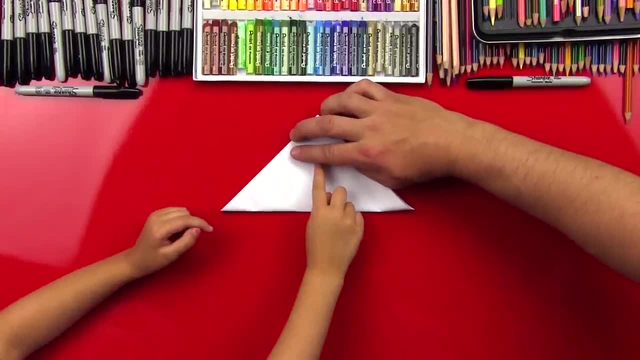 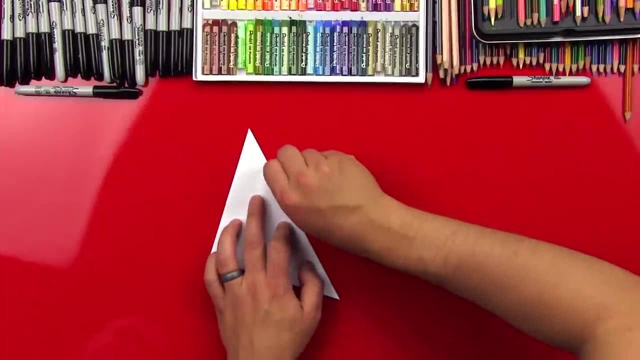 So we're going to fold down this, down this little crease here, Fold that up as far as we can go and then go ahead down the middle and then towards the edges. Perfect Little cute fingers, All right, Okay, I'm going to crease with our fingernail so it's nice and crisp. 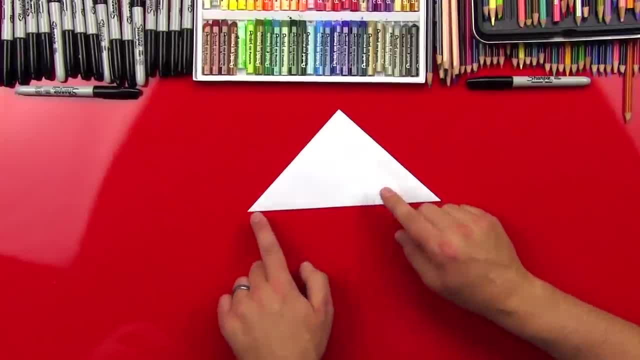 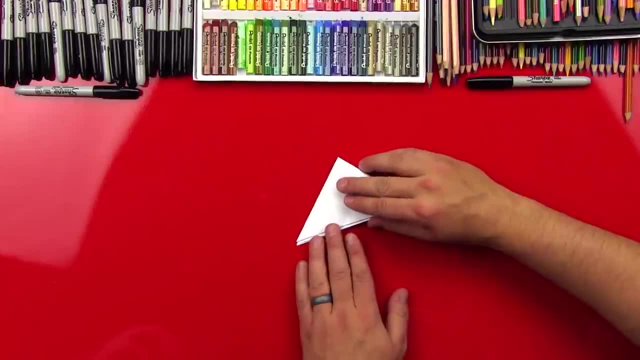 Okay, now we're going to fold it in half, So we're going to fold this corner over to this corner. Okay, Okay, All right, here we go, Fold it down, We'll line it up and you press it down. 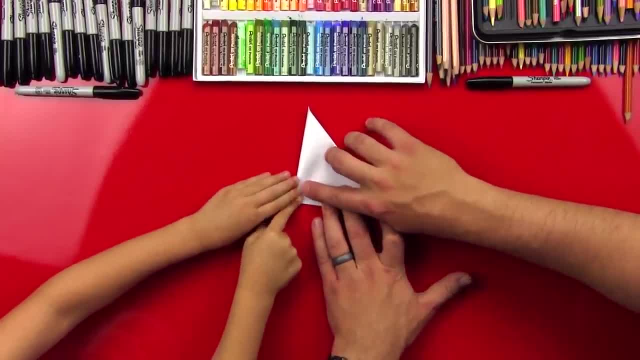 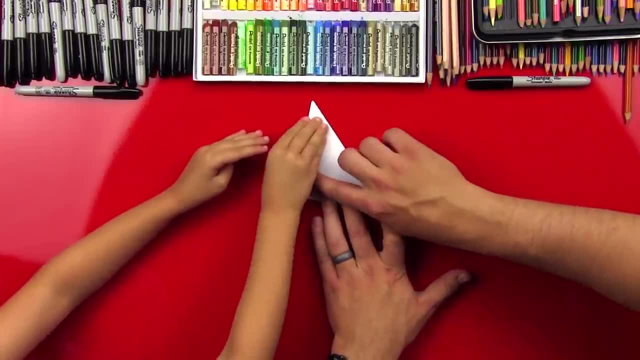 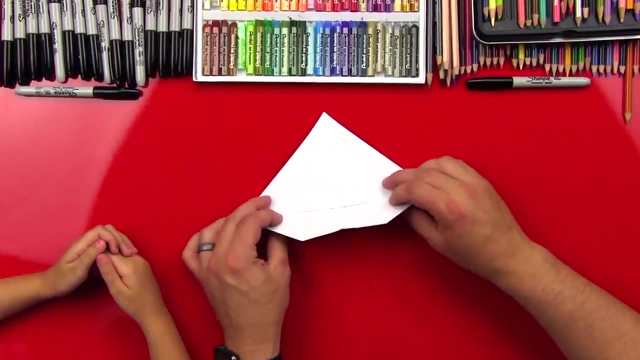 Okay, go ahead All the way down this edge. Down there, Little fingers, Use your muscles. Good job, All right. Okay, now we're going to open it back up how it was. Okay, so we got our triangle and it's folded in half. We're going to take this edge right here and we're 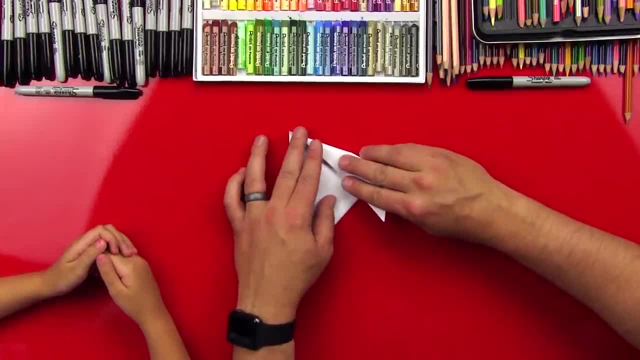 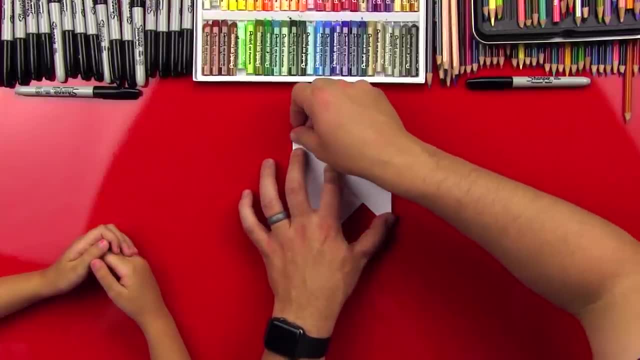 going to fold it down the middle. I'm going to fold it to the middle. So I'm going to fold it. so there's a little point up at the top And it's okay if it gets a little wrinkly because the paper gets a little thick. You want to press right there. Finish folding it. 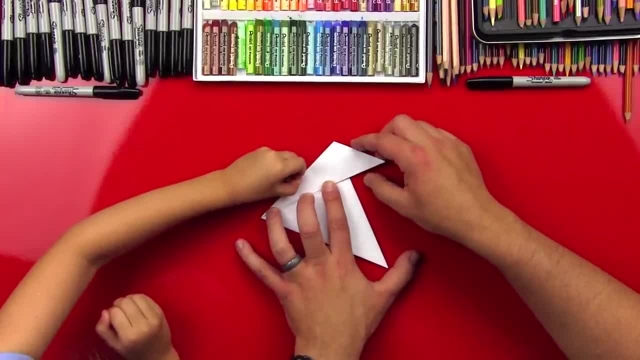 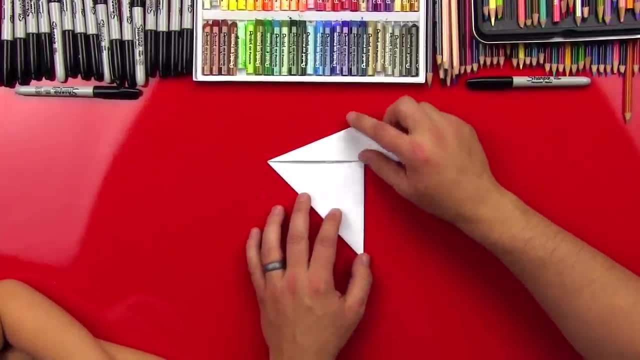 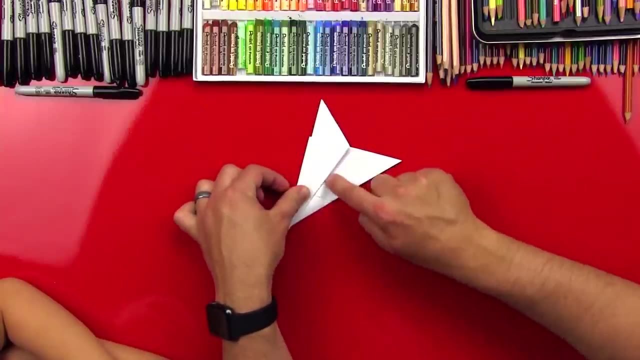 Good job, Did it? Awesome job. Okay. now what we're going to do is we're going to take this fold and we're going to fold it back, Okay, and then we're going to do another fold and fold down this line. It's almost like you're kind of rolling a burrito. Oh, now I'm hungry. 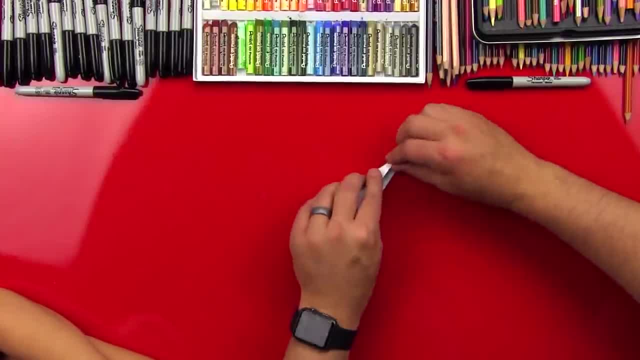 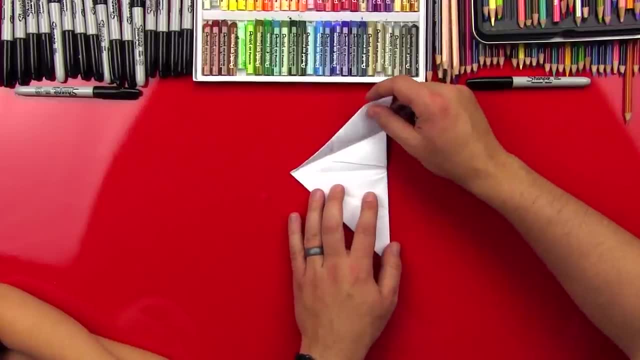 Are you hungry for burritos? No, Okay, All right, so we got that folded down, So we'll do that again. Okay, so we'll start at the beginning. So we folded this to the middle, and then we fold it again, and then we fold it one. 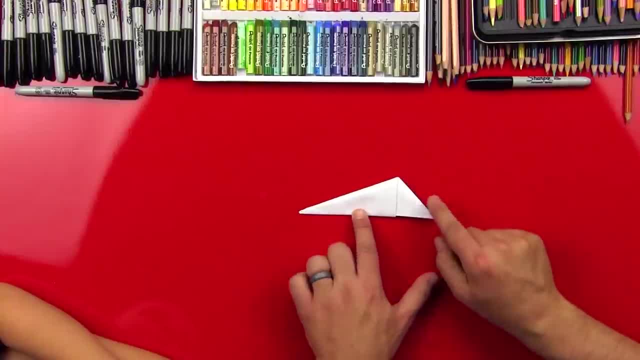 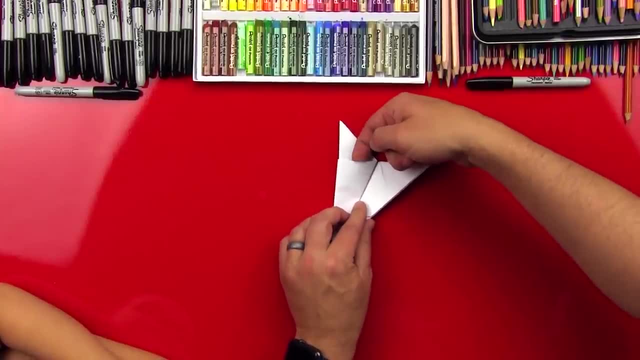 more time over like that, And so this should look like a really long triangle, right, Okay, and then we can open this back up and we're going to. there's a little pocket right here, You see that pocket. We'll put our finger in there and we can open up that little pocket. 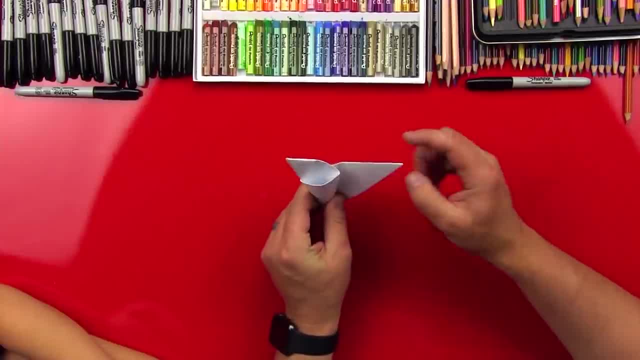 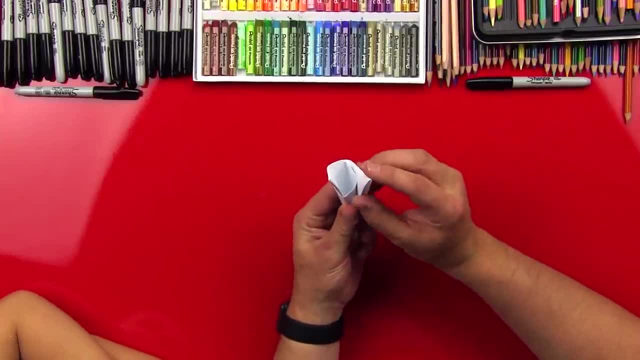 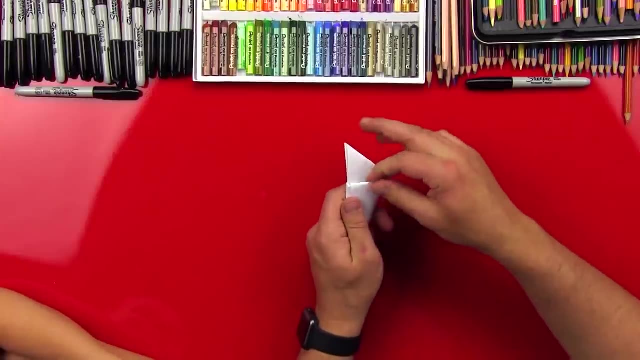 Okay, So that you can see inside it. see that, And then this corner is gonna tuck inside of there. So fold it back like this and then we can tuck that piece down inside. Not cool, That looks awesome, huh. And then we're done, because that looks like a claw a little. 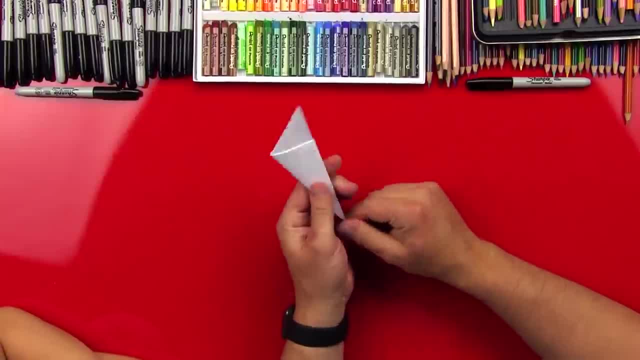 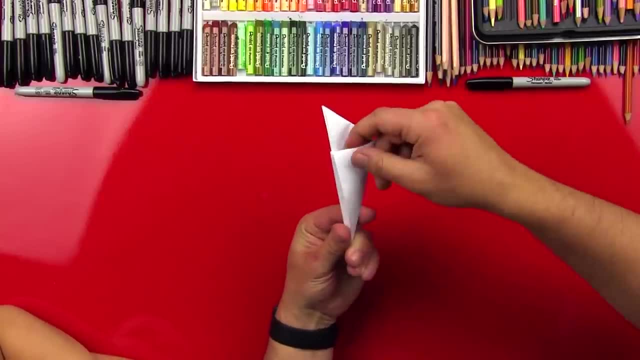 bit. So now this is how you turn it into a CLA so you can go on your finger, okay. So we'll squish it again. so opens up and that's where we put the little tab down in that pocket. and then right here there's another pocket. you see that we can put our. 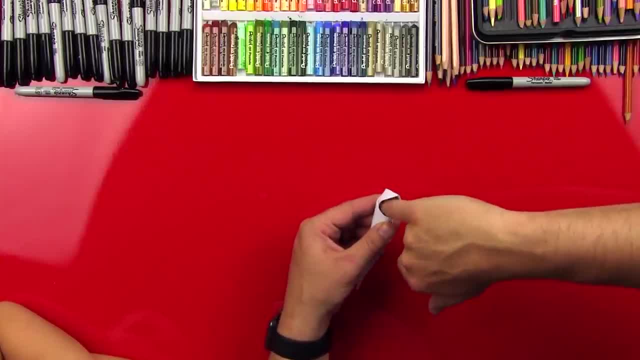 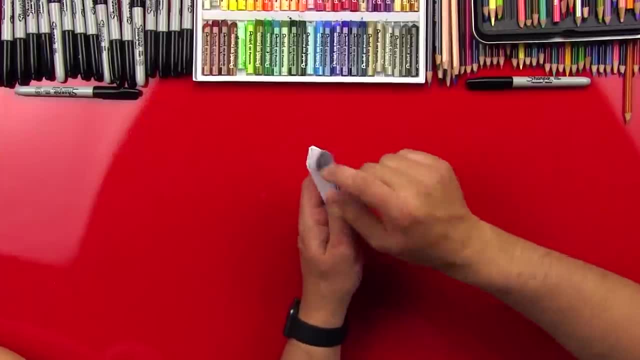 little finger inside there and open it up and then you can put your finger in there. so it's a little claw. you want to put your little figure in there? okay, let's put it in there, isn't that? awesome heads? it's pretty cool, huh? it looks like. 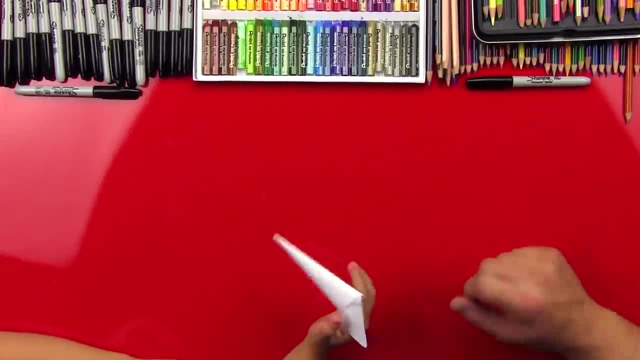 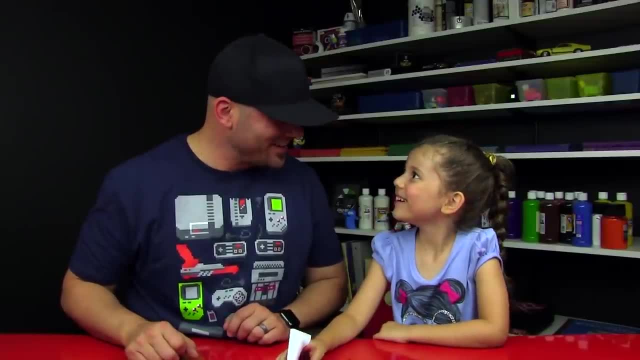 a little clock. you wiggle your finger. it looks scary, huh. so we can repeat those same steps for each one of your fingers. how many would we have to make? ten, ten, and you know what we did: make ten magically. should we put them on? yeah, all right, let's do it, let's beat it up.